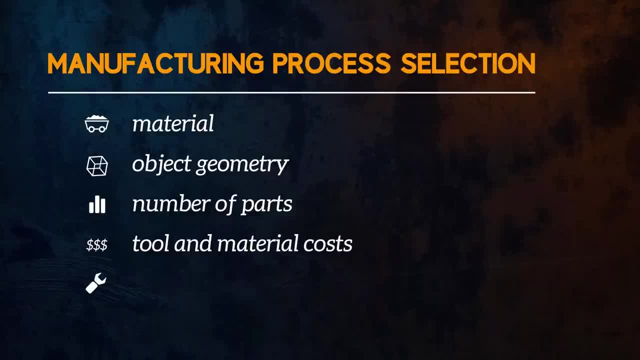 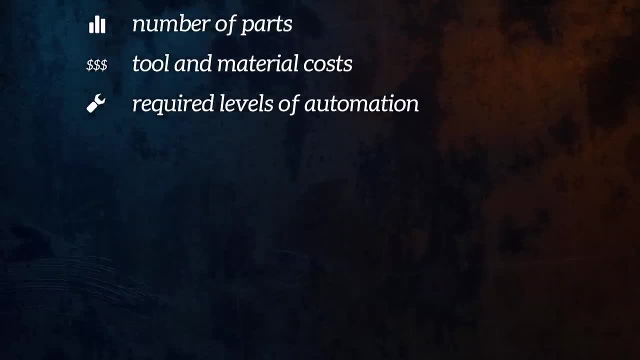 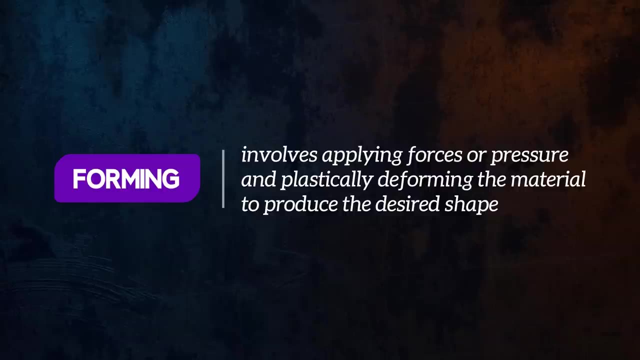 of parts you are producing, tool and material costs and required levels of automation, to name just a few. Let's look through each of the six categories in detail. Forming involves applying forces or pressure and plastically deforming the material to produce the desired shape. 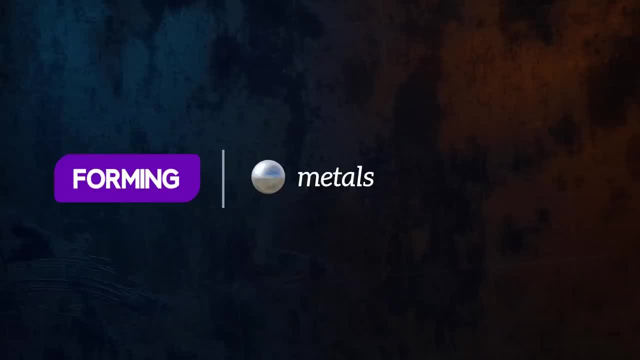 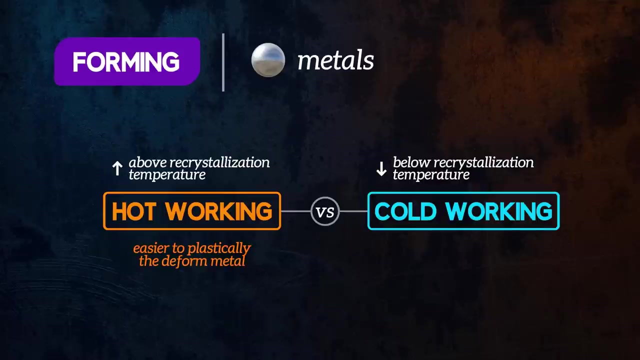 It is typically used for metals. Most forming processes can be done when the metal is either above or below its recrystallization temperature. This is known as hot or cold working. Hot working makes it easier to plastically deform the metal, But cold working causes strain hardening, which increases the strength of the material. 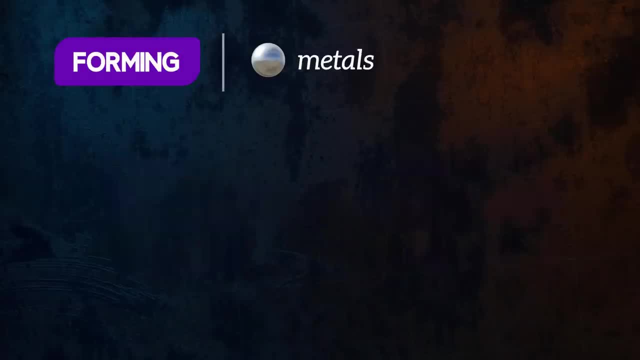 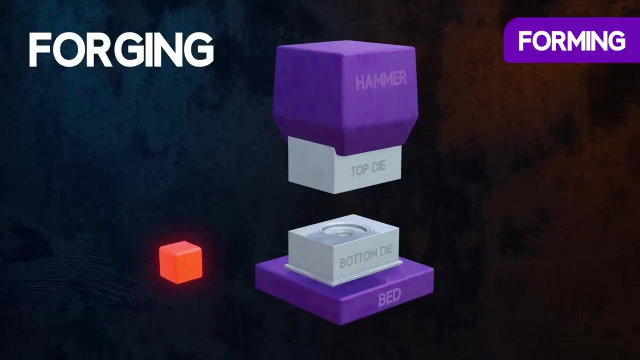 This is a very common process. Three common forming processes are forging, rolling and extrusion. Modern forging is done using machines, Enclosed die or impression forging. The metal is placed between top and bottom closed dies. Repeated strokes from the hammer are used to cause the metal to flow into the shape. 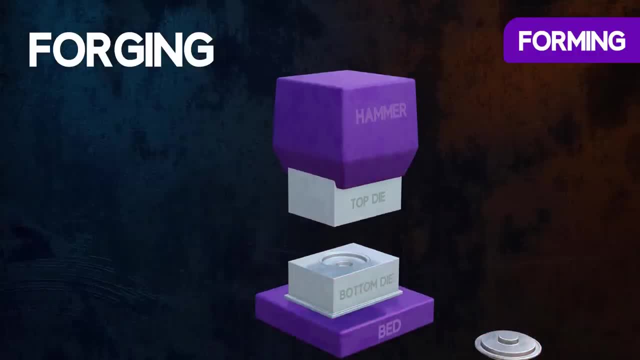 of the dies. Objects produced using forging can have improved mechanical performance. The metal is then placed between the top and bottom closed dies. Repeated strokes from the hammer are used to cause the metal to flow into the shape of the dies. The metal is then placed between the top and bottom closed dies. 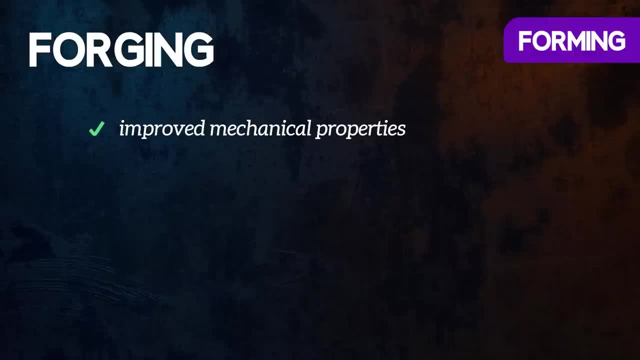 The metal is then placed between the top and bottom, closed dies Aceeding. such 저기 practice is an important by Canadians zum. hurtings will only be slightly fewer in our world than would be possible in the US. The Pardon for Ch veins Drᵒ stone International. 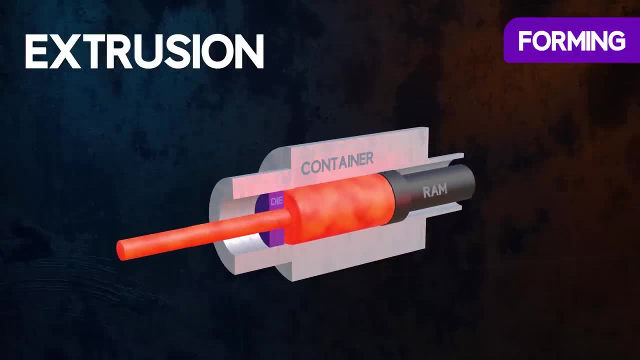 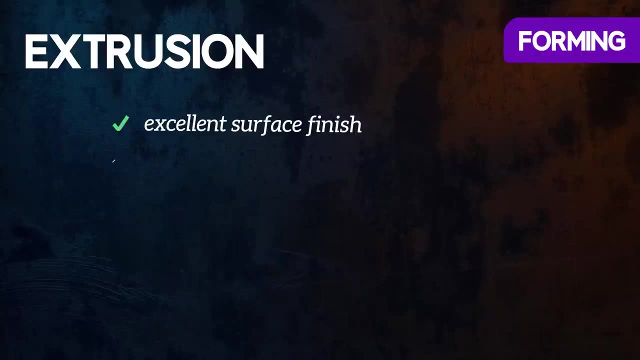 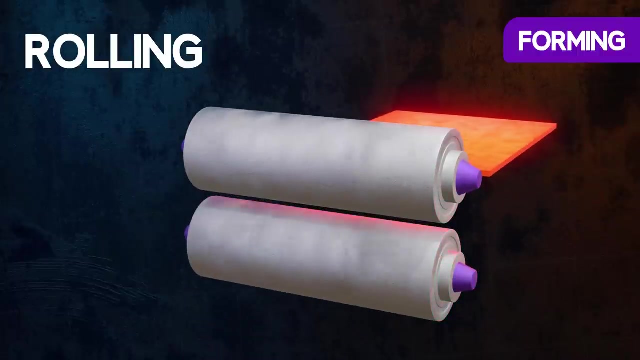 mund order Utility 구두. external. collecting the building. free about the, but it is only suitable for producing two-dimensional shapes. Rolling is probably the most commonly used forming process. It involves passing metal between two or more rollers, which apply pressure and reduce thickness. 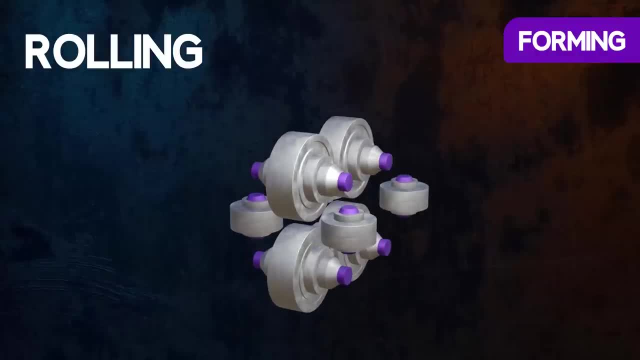 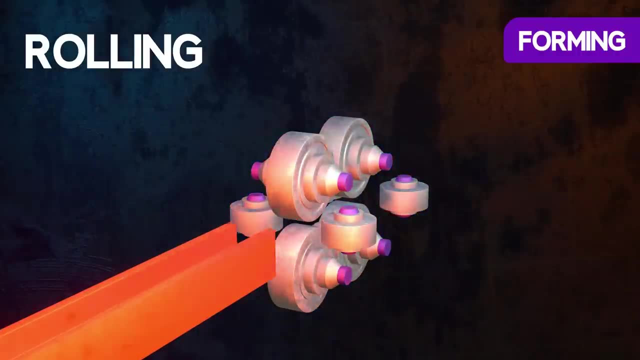 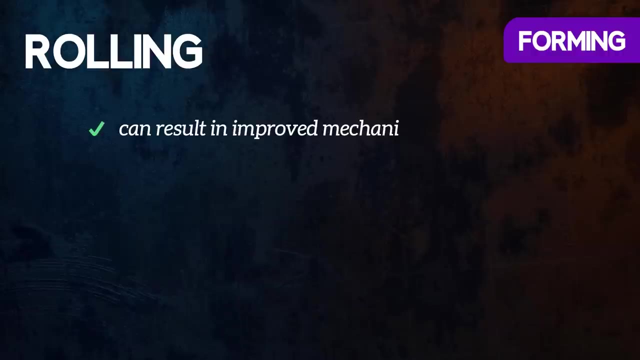 More complex products like I-beams can also be manufactured by rolling. Rolling can result in improved mechanical properties and can be automated, which makes it good for large-scale production, but tooling costs tend to be high and it can't be used to produce very complex shapes. 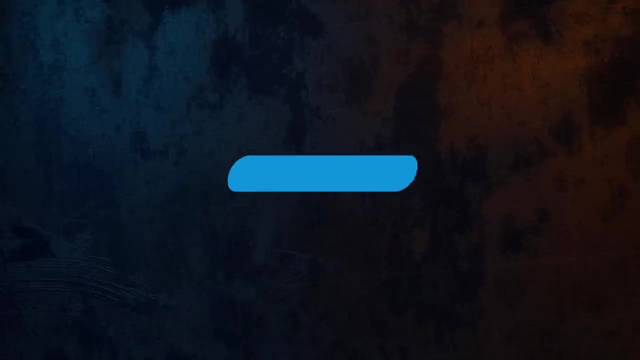 Let's move on to the next category of manufacturing processes. casting Casting involves pouring molten metal into a mold and allowing it to solidify. It is what we call a primary shaping process. a secondary process, such as machining, is typically needed to achieve the desired surface finish. 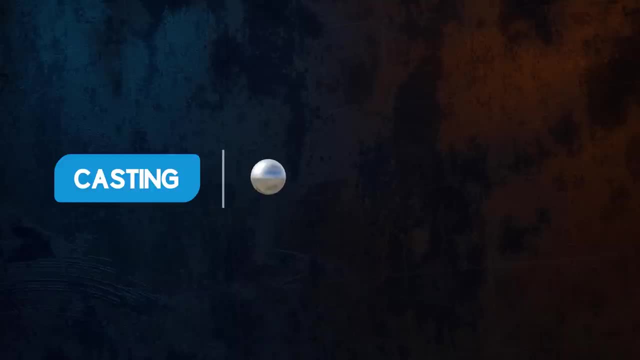 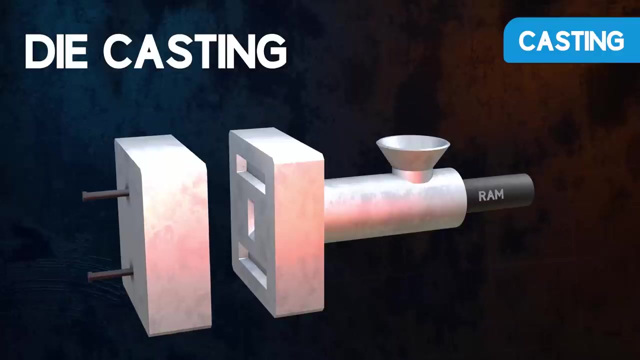 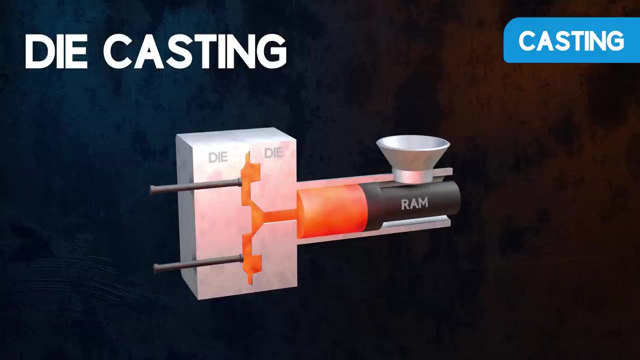 Like forming, casting is most commonly used for metals. Three common types of casting are die casting, sand casting and investment casting. In die casting, molten metal is forced into reusable metal dies at high pressure. Once the molten metal has solidified, it is removed from the mold. 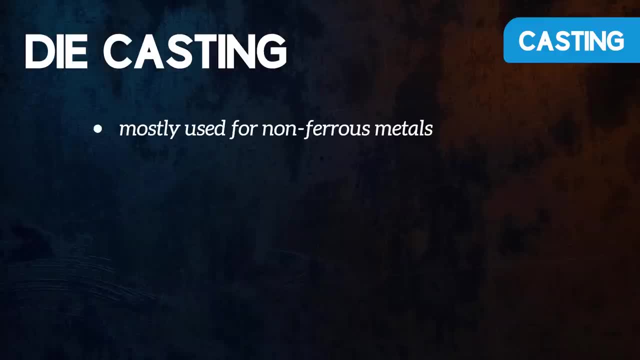 Die casting is mostly used for non-ferrous metals like aluminum and zinc, which have low melting temperatures. It provides an excellent surface finish and can achieve very tight tolerances, but startup costs tend to be high, so it is only really suitable for large production runs. 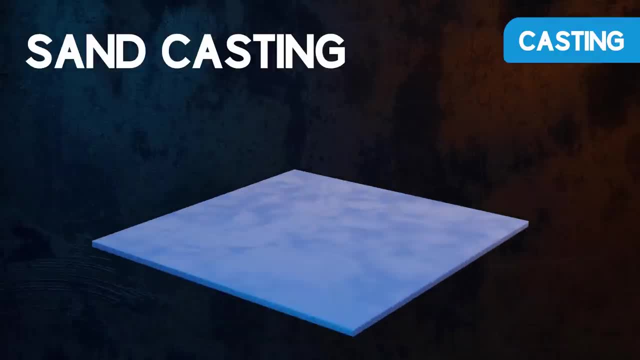 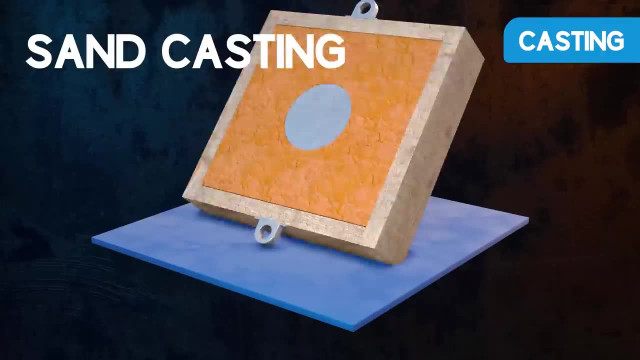 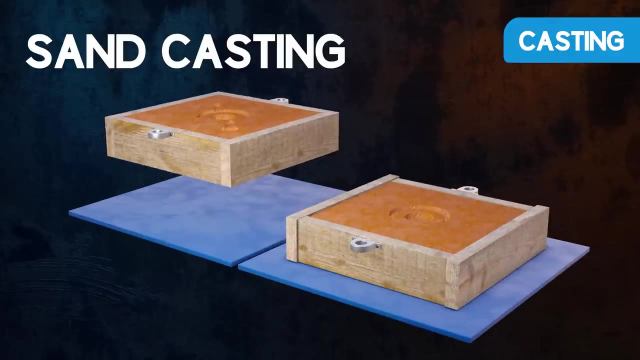 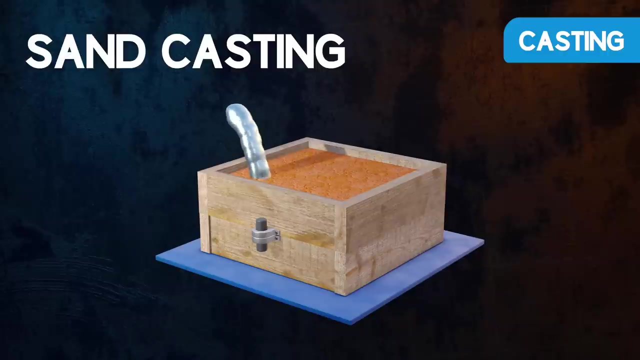 In sand casting, a pattern is used to create a single-use mold from damp sand. The sand is typically contained in two mold boxes called the cope and the drag. Molten metal is poured into the mold through a channel formed in the sand. When the metal has solidified, the cast object can be used to create a mold. 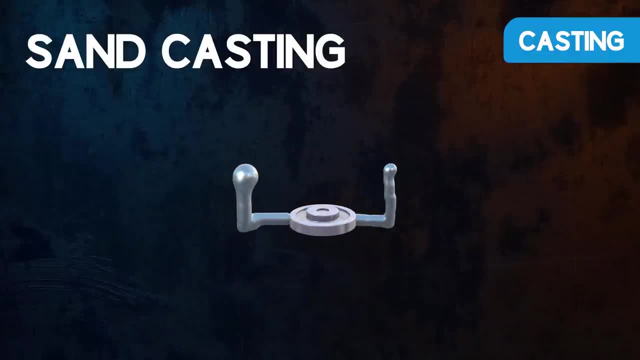 When the metal has solidified, the cast object can be used to create a mold. When the metal has solidified, the cast object can be used to create a mold. The cast object can be removed from the sand. Sand casting can be used for a wide range of metals. 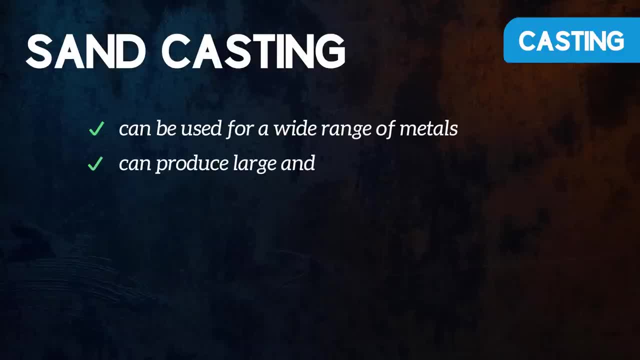 including those with high melting temperatures. It can produce large and complex parts and initial costs are very low, making it good for small production runs. However, it provides a poor surface finish and is not as accurate as other casting processes. The last casting process we will look at is investment casting. 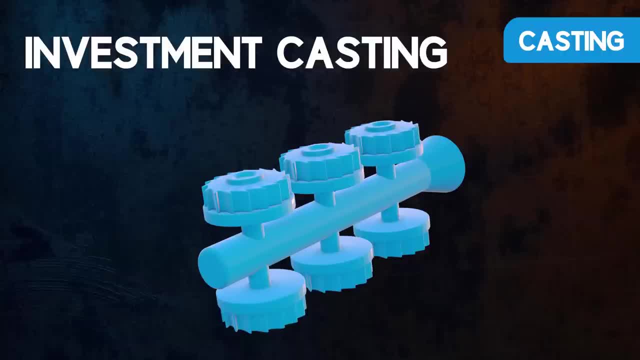 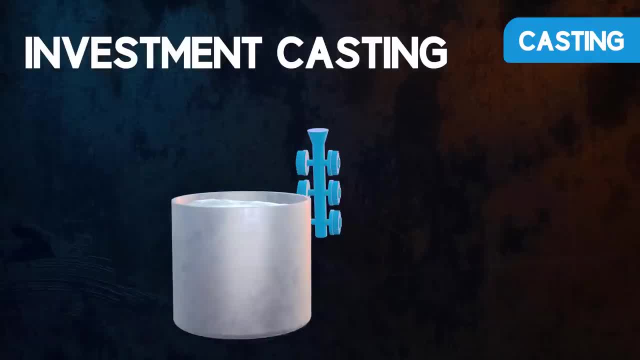 will be used to 문제 bard like healing or wounding your head. Most wax pieces will be cast into flavour dessa. Most wax pieces will be cast into flavour. tässä, The wax tree is dipped into a slurry to create a ceramic mold. 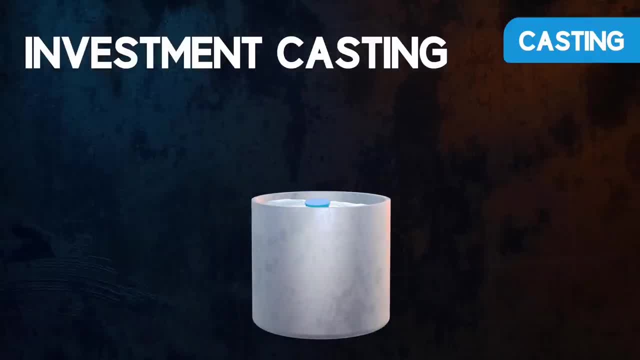 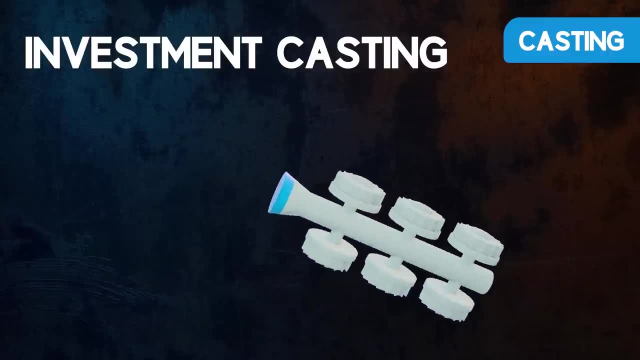 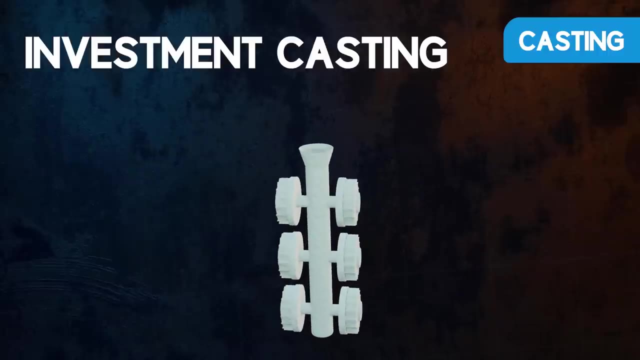 match 24 lots per unit. Heat is applied to melt out the wax. Molten metal is then poured into the ceramic mold pour in. has cooled, the mold is broken off. Investment casting is good for parts with complex geometry and can achieve tight tolerances. 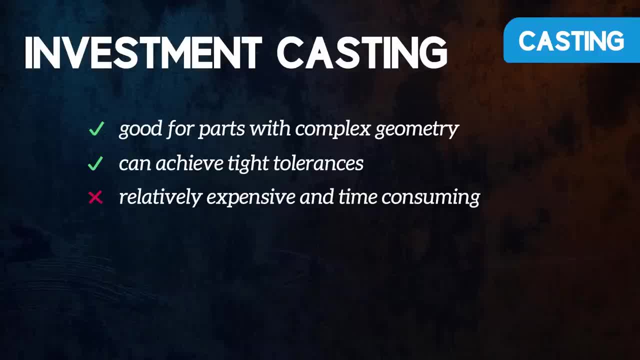 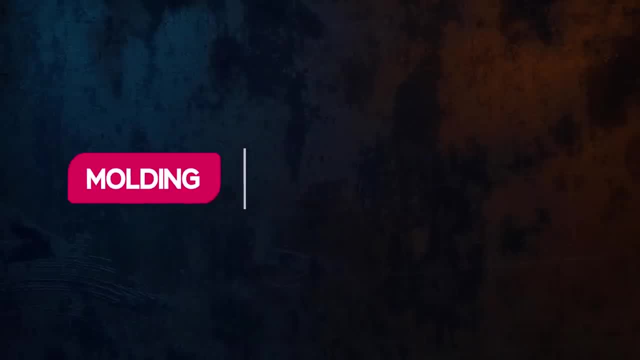 but it is an expensive and time-consuming process. Molding is very similar to casting. It involves shaping a liquid or pliable material using a mold. Most of the time, molding is used for forming plastics. Typical molding processes are injection molding, compression molding and blow molding. 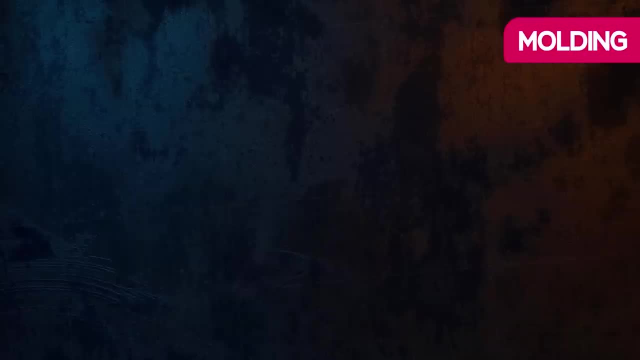 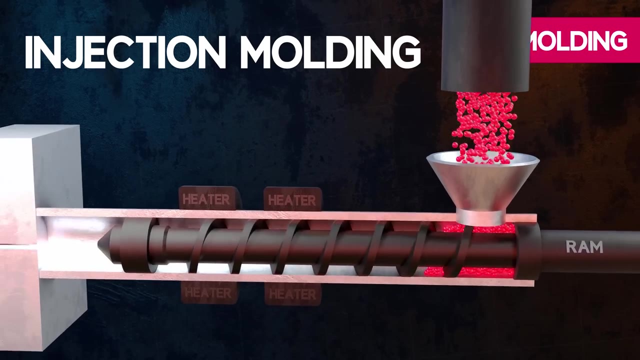 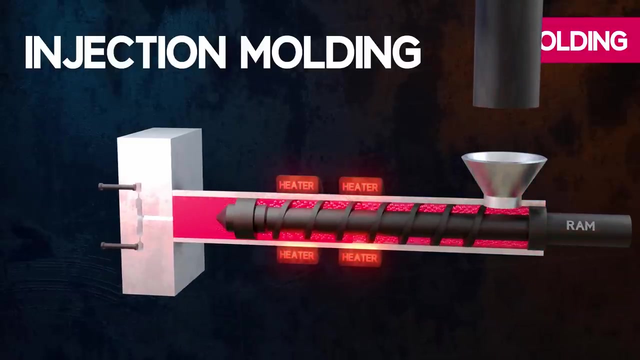 Let's look at the first two. Injection molding is the most commonly used manufacturing method for plastics. Polymer granules are fed into the hopper and a screw is used to pass the material through a heated cylinder before it is forced at pressure into the mold. 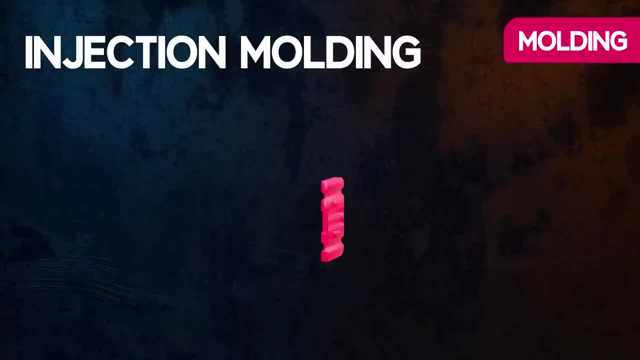 Injection molding is also used for molding. Injection molding is mostly used for thermoplastics, which are polymers which soften when they are heated and harden when they are cooled. It is a very fast process and can be fully automated, meaning labor costs are low. 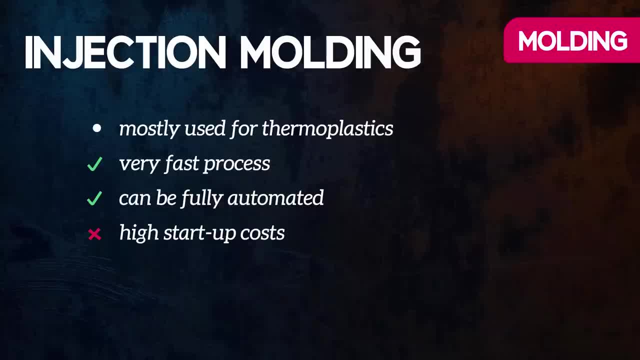 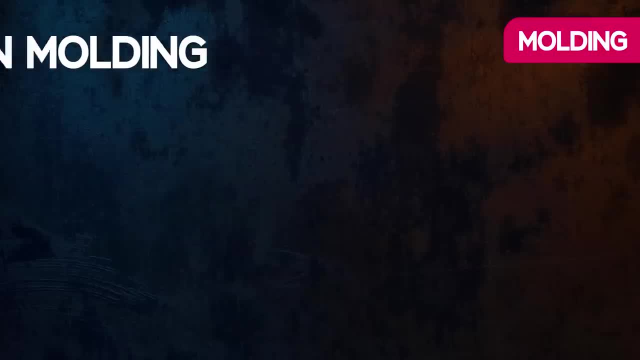 But startup costs are very high due to the expensive molds, so it is really only cost effective for large production runs. Injection molding is used for molding. Compression molding is used for molding. Injection molding is used for molding. Injection molding is mostly used for thermoplastics, which are polymers which soften when they are. 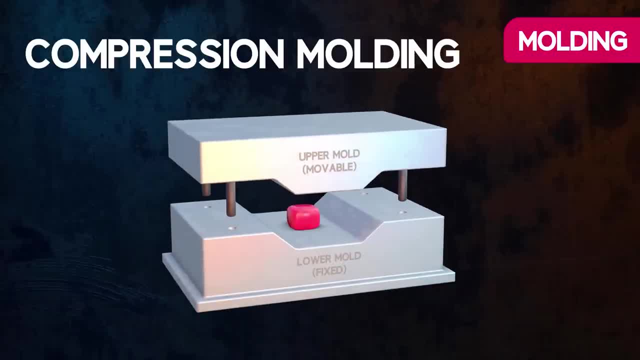 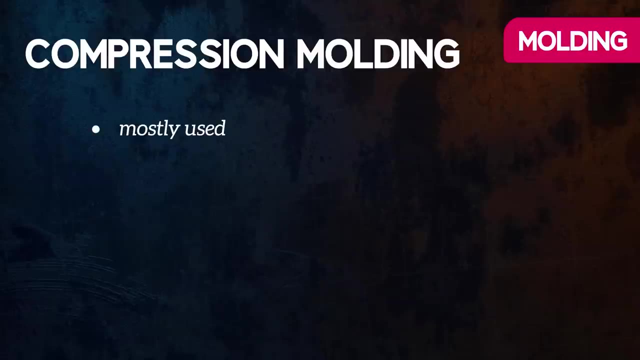 placing a precise amount of material into a mold. The mold is closed and pressure and temperature applied. Compression molding is mostly used for thermosets, which are polymers which irreversibly harden when heated. Tooling costs are relatively cheap, making it good for small production runs, but it 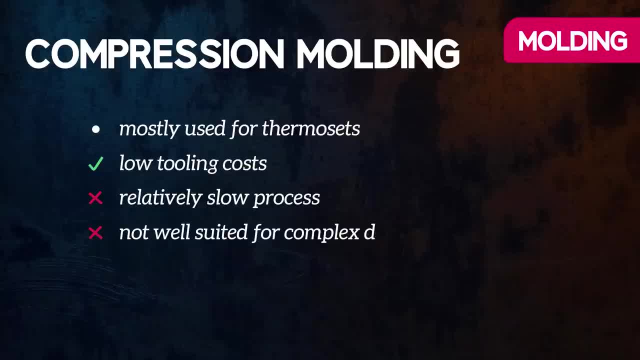 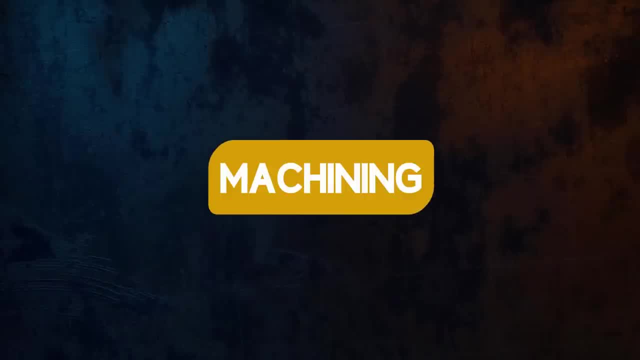 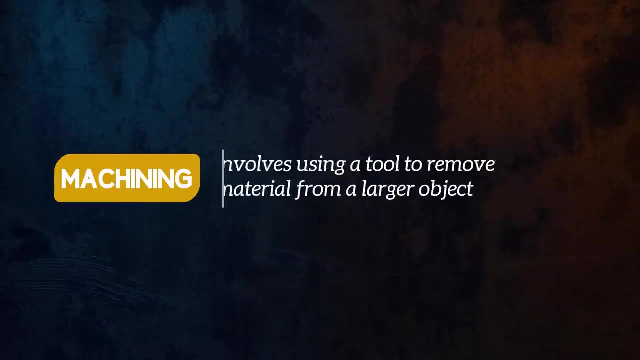 is quite a slow process and is not well suited for complex designs. So far, we have only looked at material deformation processes. Machining is a material removal process where a tool is used to remove material from a larger object. It is often used for secondary shaping, when the part has already been formed using a primary. 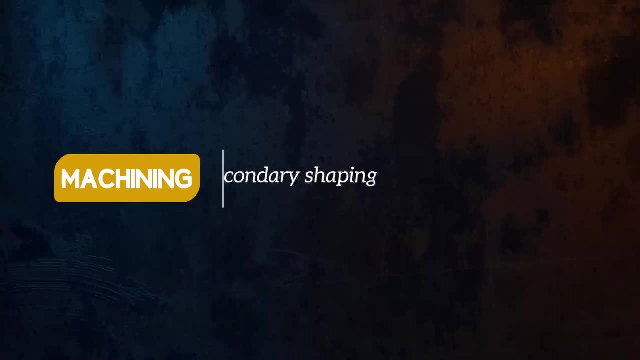 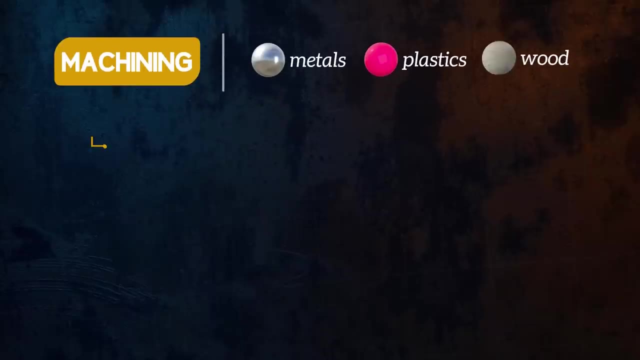 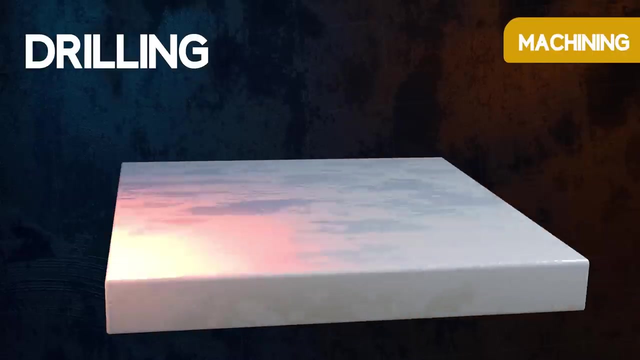 process like casting. Machining can be used for a wide range of materials, including metals, plastics and wood. Examples of machining include drilling, turning and reaming. Drilling is the cutting of a normal circular hole by pressing a rotating drill bit through. 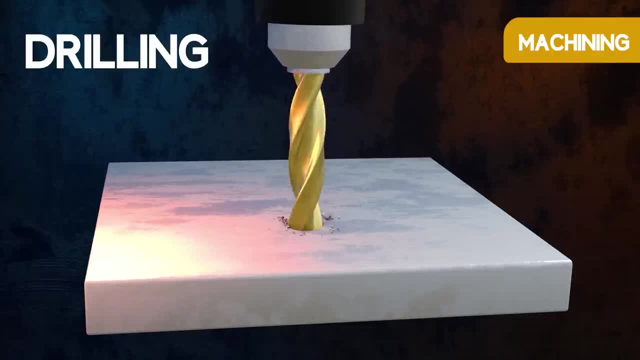 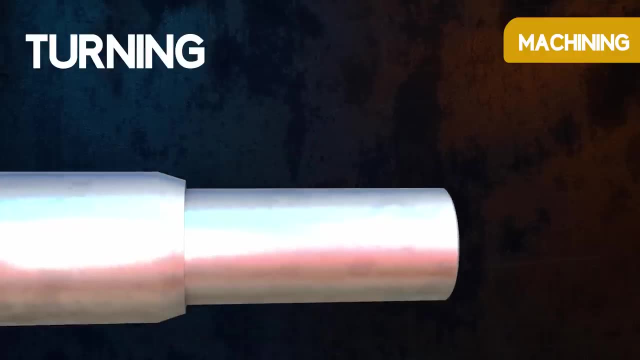 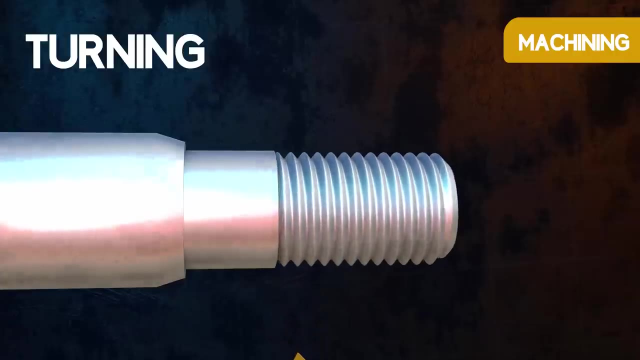 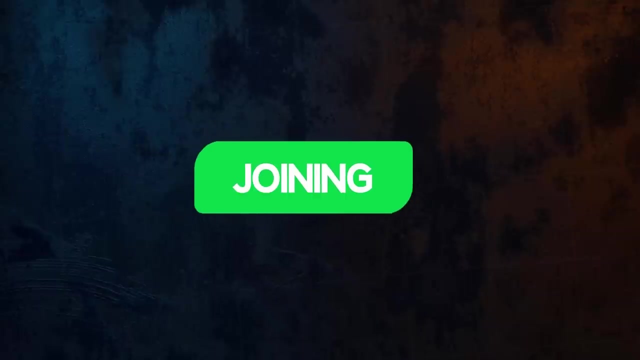 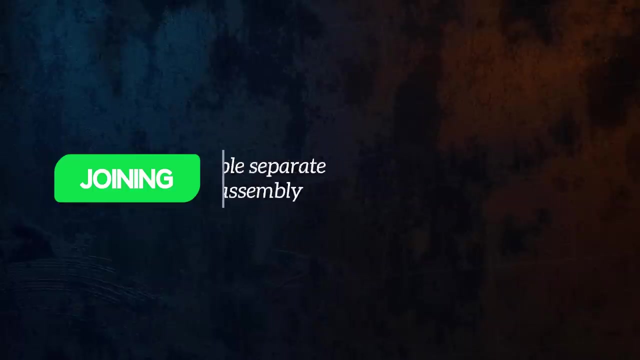 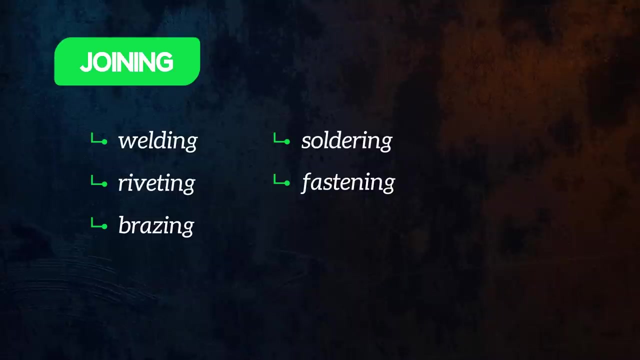 a solid object, And turning is the use of a cutting tool to shape a rotating workpiece. Let's move on to the next category. Joining involves combining multiple separate components into a larger assembly. Like machining, joining is a secondary process. Welding, riveting, brazing, soldering and fastening are all different types of joining. 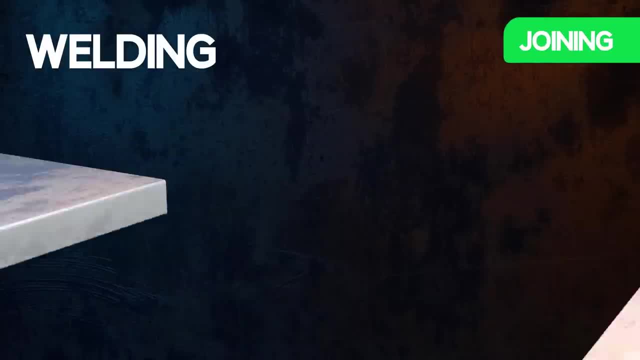 processes. Welding uses extremely high heat to fuse distinct metal parts together. The jointing process is a process that requires a lot of work. The jointing process is a process that requires a lot of work. The jointing process is a process that requires a lot of work. 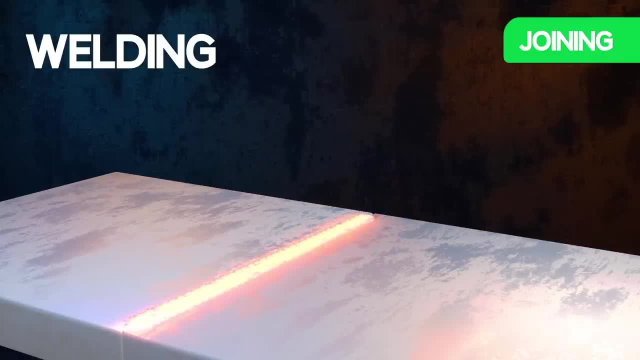 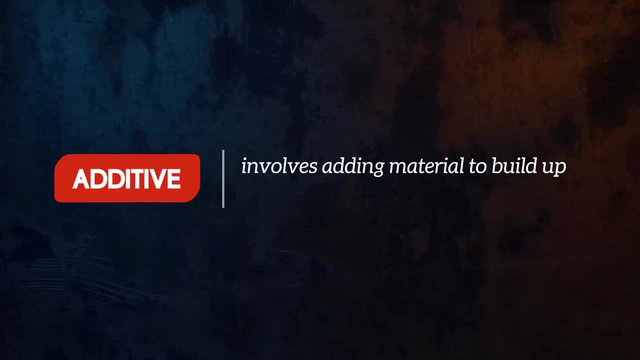 Unlike soldering and brazing, the base metal melts during welding. The final category is additive manufacturing, which involves adding material to build up the desired object, typically one layer at a time. 3D printing, selective laser sintering and vat polymerization are examples of additive. 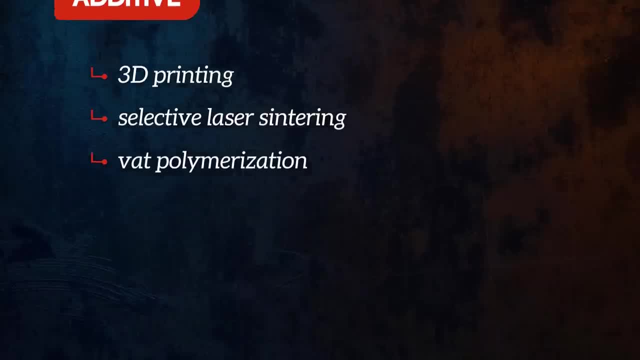 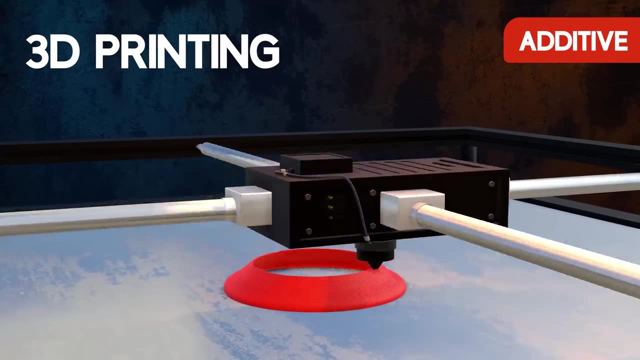 manufacturing techniques. 3D printing is a process that requires a lot of work. In 3D printing, a computer is used to successfully build up an object layer by layer. 3D printing is a slow process and the range of materials which can be used is limited.